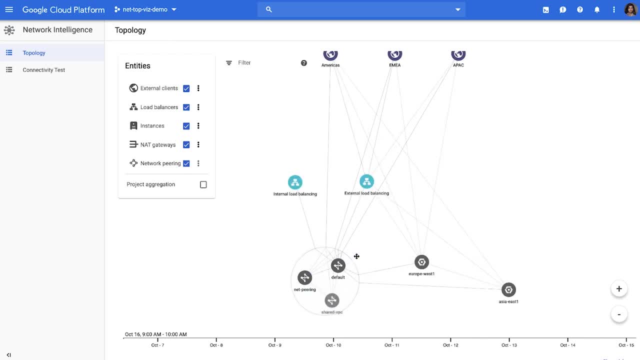 they're deployed in. You can drill down to the specific VM instance level as needed. Many customers want to use this to quickly verify certain policies. For instance, let's say you have a policy in which all the traffic should be going through the load balancers. You can click on the. 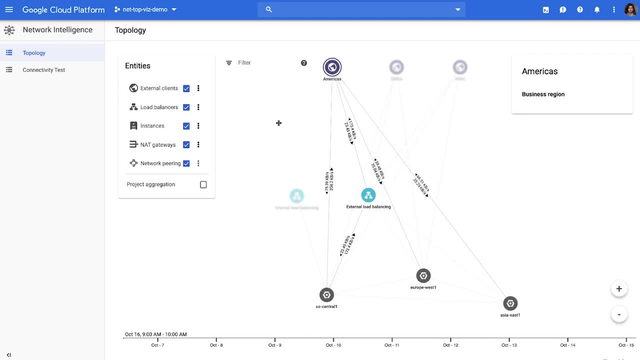 region or an external geo region to see all the traffic and verify the policy. Here you can see that there is some traffic going directly from a GCE instance to the internet. Another example of a common use case for customers is to proactively verify if the traffic is being served out of the 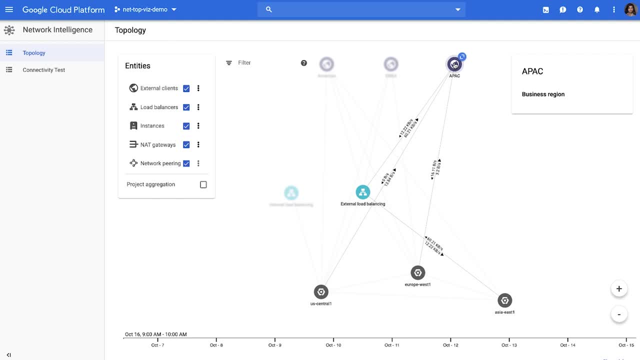 optimal region. For instance, here you can see that the APAC clients are being predominantly served out of the Asia East region. This would help you troubleshoot performance issues that may happen as a result of traffic being served out of a non-optimal region. 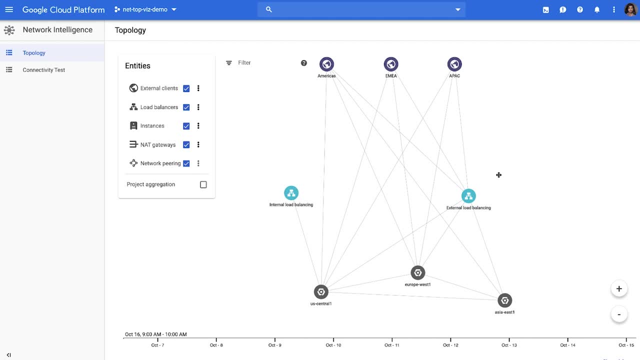 You would be able to easily see which regions the traffic is being served out of. You can also see the evolution of topology by going back in time by clicking on this timeline on the bottom. This is very useful in several scenarios, For instance, if a network event happened. 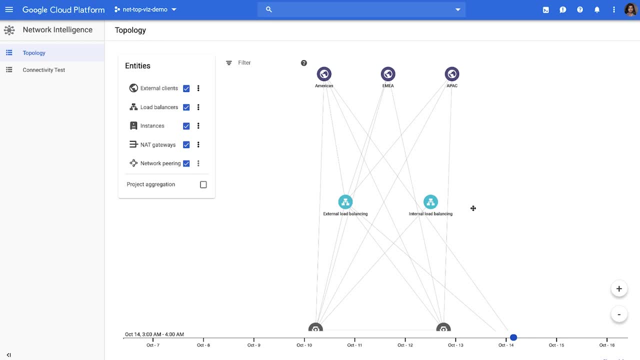 and you want to troubleshoot it. you can look at the topology around the event using this capability to determine any topology changes. you may have contributed to the network issue During migration. it helps you to monitor the state of your deployment as you migrate your workloads. 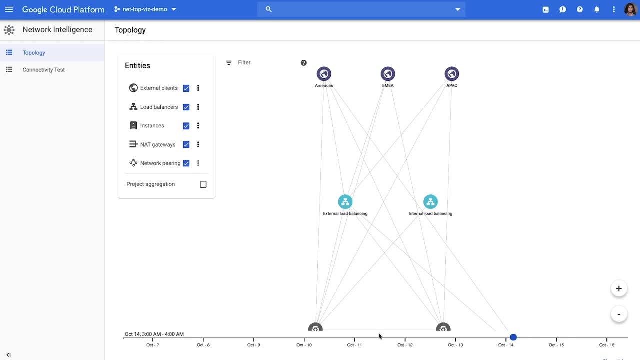 thus providing better visibility into your migration process and also letting you track it by looking at the topology evolution through time. For troubleshooting, the search capability is very helpful, For instance, if you wanted to search for a specific instance and see what all it was talking to. 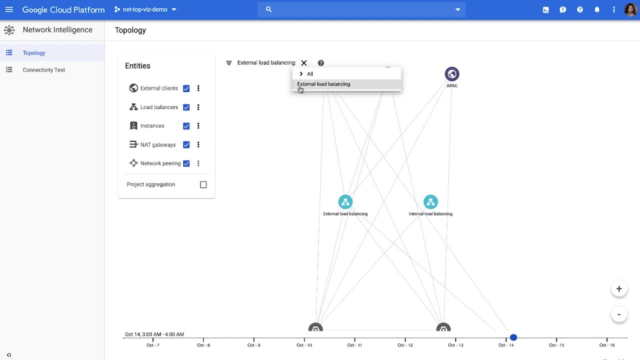 or a specific load balancer. you can do all those kinds of search using this capability. That way you can drill down into exactly what you're searching for. All edges in the visualization have metrics associated with them. You can click on any edge and view. 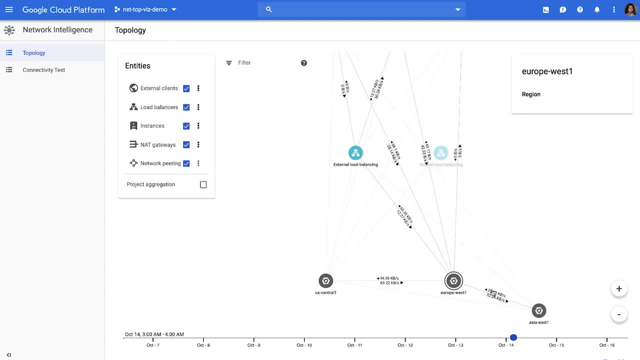 how the metric changed over a period of time. You can see throughput in these metrics- ingress and egress, byte counts and others for monitoring your network health. If you have VPC flow logs available and you want to drill in more to analyze those logs,